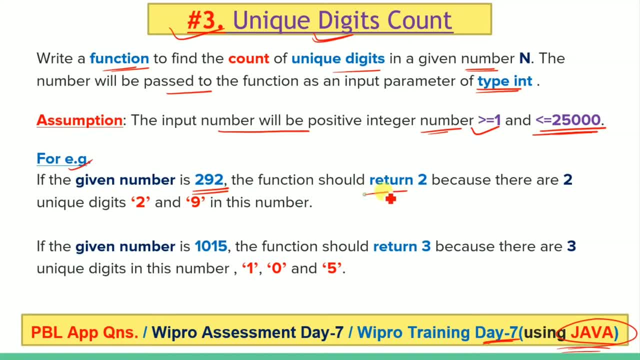 if the given number is 292, then the function should return 2, because here we can see that there are two unique digits, that is, 2 and 9, in this number. and the another example is: if the given number is 1015, then the function should return 3, because here we can see that 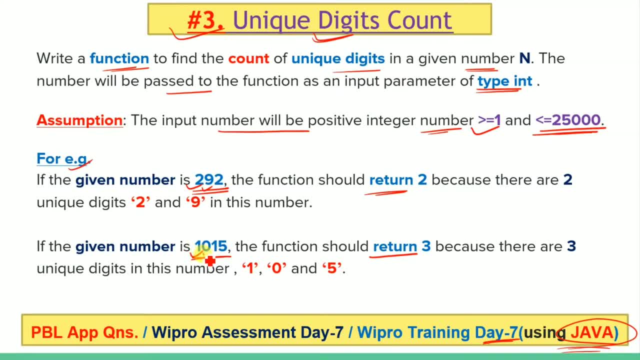 there are three unique digits, that is, 1, 0 and 5.. So we will write the problem For this question on visual studio code. So before I start, please subscribe our channel to get all the questions and solutions of vpro training. So now let's open visual studio code. 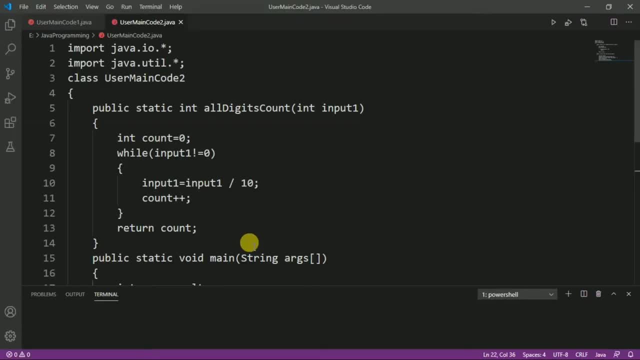 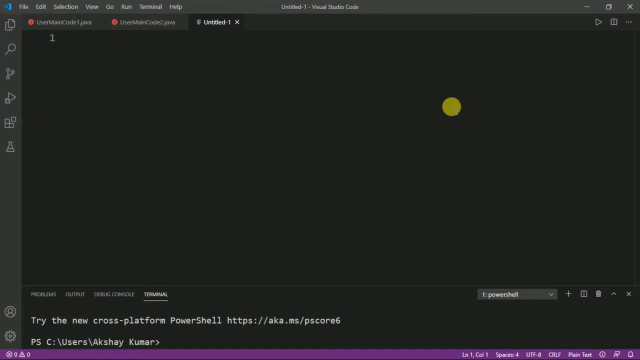 and press control n for new tab. At first we will write the program. after that we will see how it works. So initially we have to import some java packages, so that we have to write import javaiostar and the another package is import javaiostar. 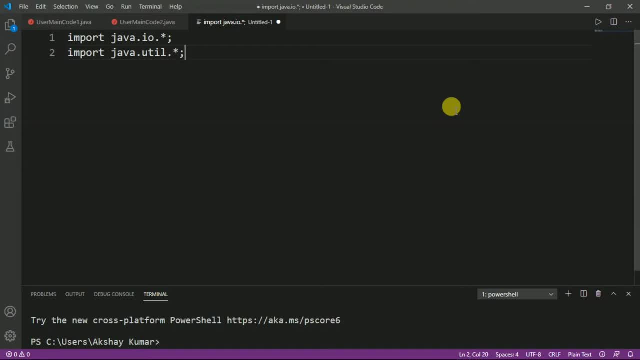 And now we have to define the class name. So let's give the class name as user main code 3, because this is our third question of day 7. and now by pressing control s we will save the program, and here our program name should be same as the class name. So here we have to write same. 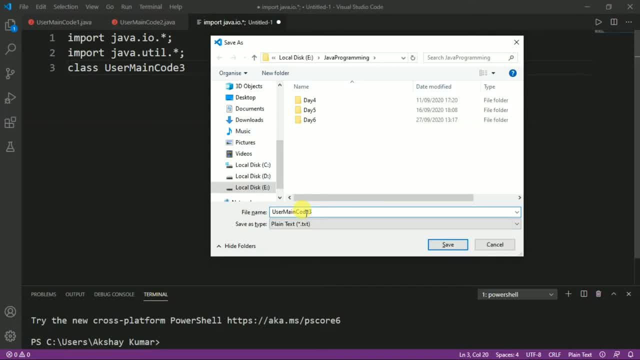 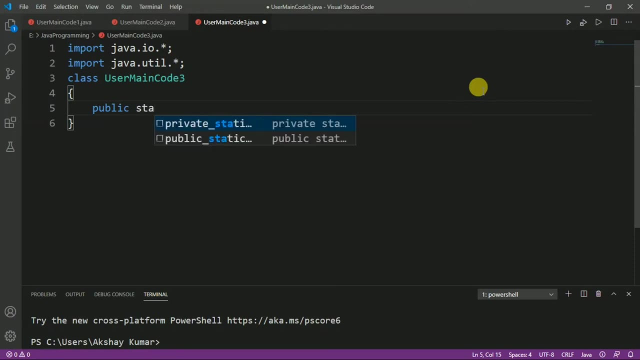 as user. main code 3 with a extension dot java. And now we will select all files and let's save. and now we will define the function so that we have to write public static int. Let's give the function name, as unique digits count, and we will take one formal argument as an input, that is input 1. after that we will declare: 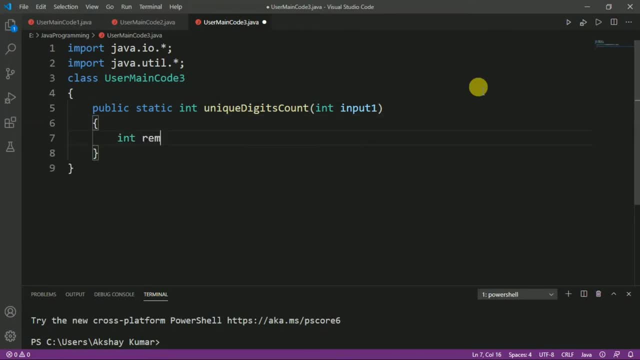 some variables, So let's take. So let's take rdm for reminder, and we will initialize it to 0. and we will take another variable as count, and we will also initialize it to 0.. Count is for counting the unique digits and after that we will write the condition for. 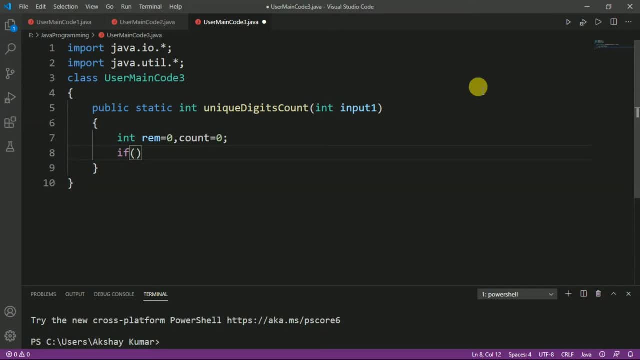 taking the number which is greater than or equal to 1 and less than or equal to 25000.. So here we have to write: input 1 is greater than or equal to 25000.. Our input Guess is 0.. And input 1 is less than or equal to 25000. 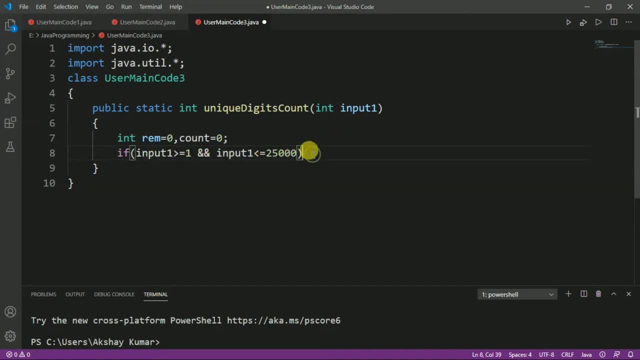 Our number should be in the range 1 to 25000, and after that we will take the array of size 10, so that we have to write int arr equal to new int of size 10.. And, uh, So, now that I have, by now, vezes 10 in size 10.. 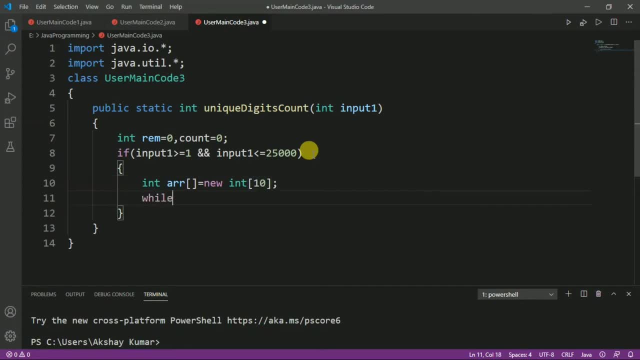 I will take x. you will see that we will take while loop and we will write the condition. while input 1 is not equal to 0, then we will perform the operation. remainder equal to rdm, equal to input 1 modulus 10. so we have to write input 1 modulus 10 and after that we will take the condition if arr of remainder. 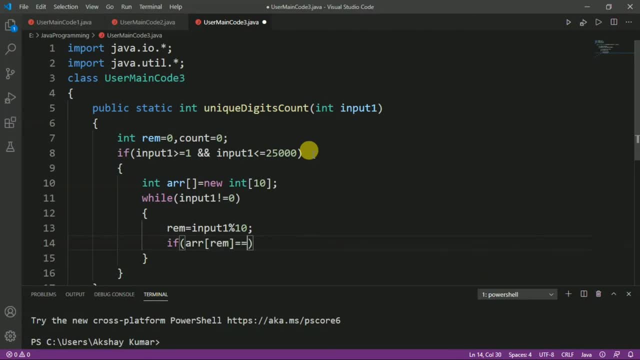 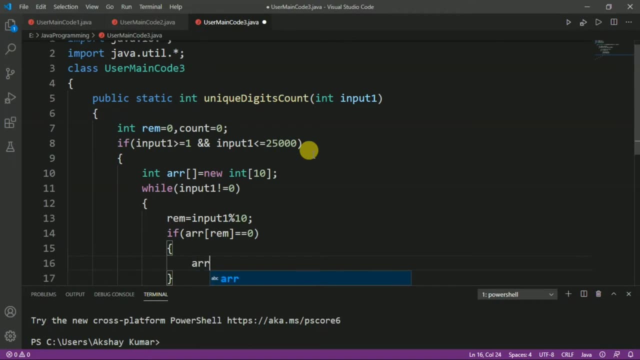 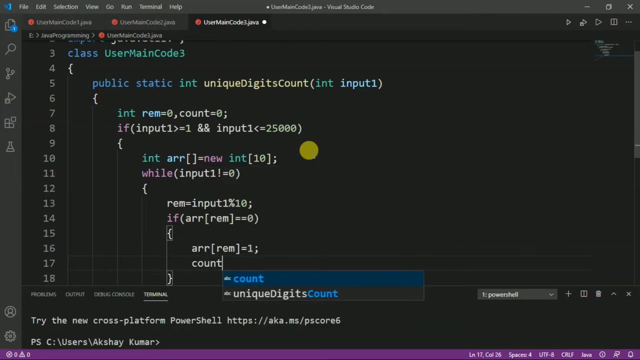 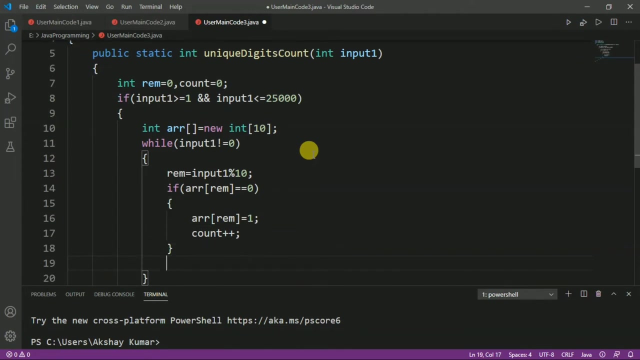 equal to equal to 0, then we will perform the operation which is arr of remainder equal to 1 and after that we will increment the count and outside, if block, we will write the operation: input 1 equal to input 1 divided by 0.. 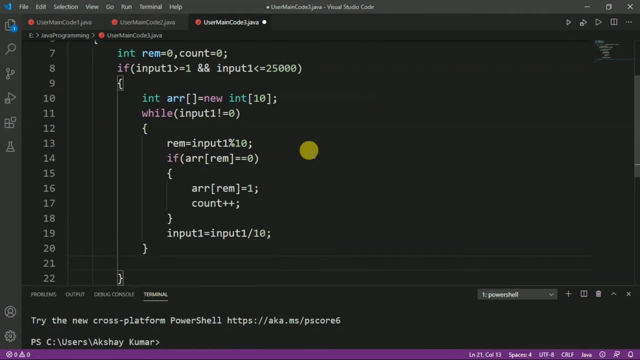 10, and outside while loop we will return count and after that outside, if block, we will return 0. now we will write the main function here, so that we have to write public static void main, and here we will pass the string args and after that we will declare some variables, so that let's 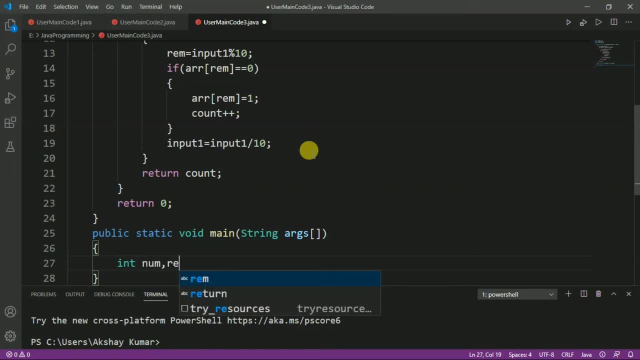 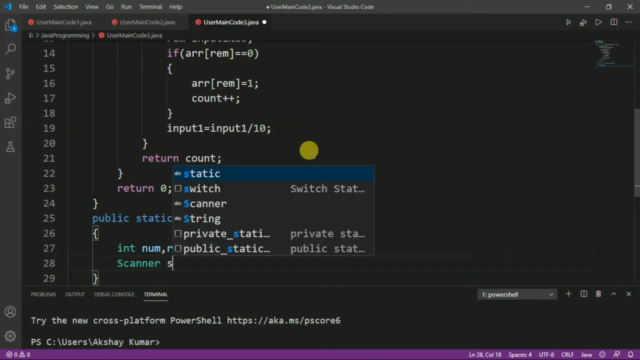 take nvm4 number and we will store the value of calling function in the variable result. now we will create the object of a scanner class, so that we have to write a scanner as c equal to new scanner, and here we will pass the system dot in which will represent the keyboard, and after that we will take 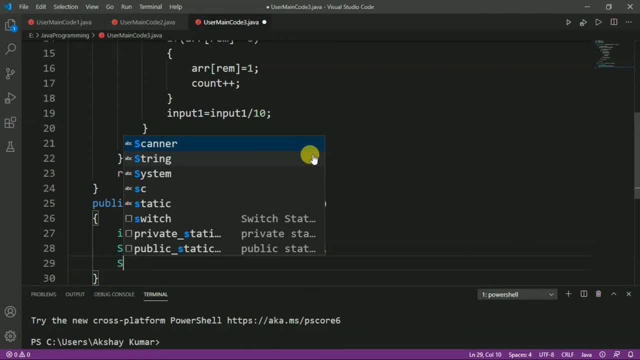 the input from user, so that we have to write the message to the user to take the input, so that we will write system dot sect out dot println, and here we will write the messageそして nvm4, Enter the number, and after that we will read that number from keyboard and we will restore that into the num variable. so we 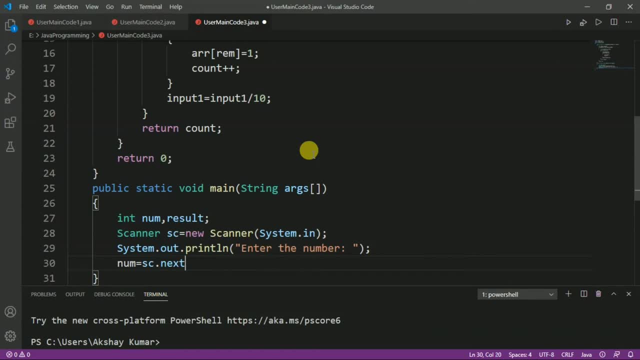 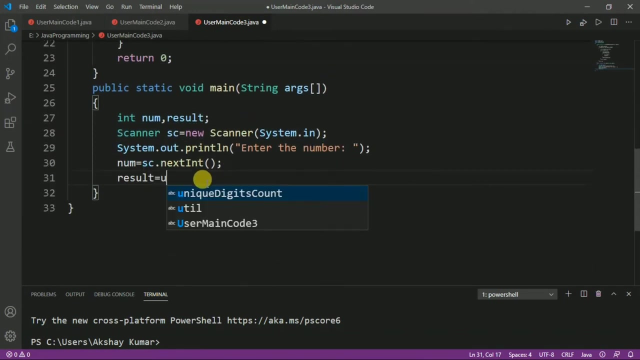 have to write num equal to our function. name is unique digits count. so here we have to write same as unique digits count, and now we will pass the actual argument that is stored in the num variable. so here we have to write num, and now we will print the value. so 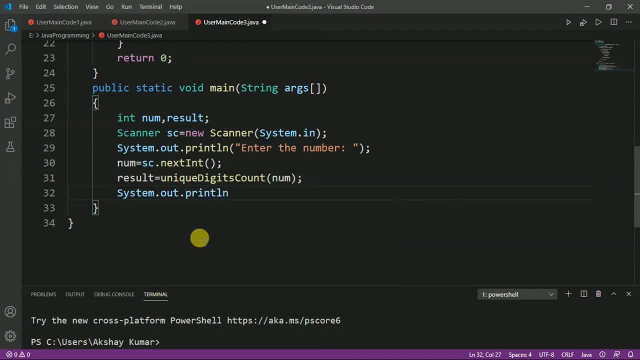 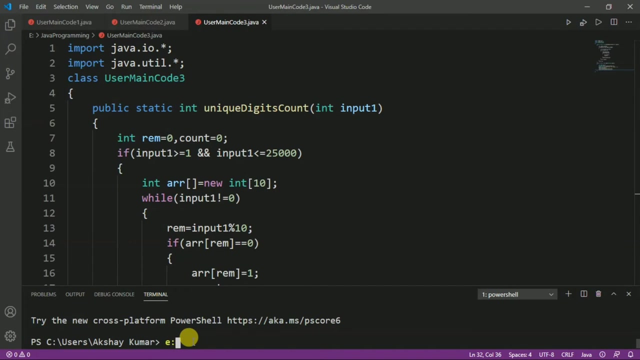 let's write system dot, auth, dot, println, and here we will pass the variable result, and now by pressing ctrl s we will save the program, and after that we will run the program. and before run this, let's go into the drive where we have saved our program, and in my case I have saved my program in the drive e in. 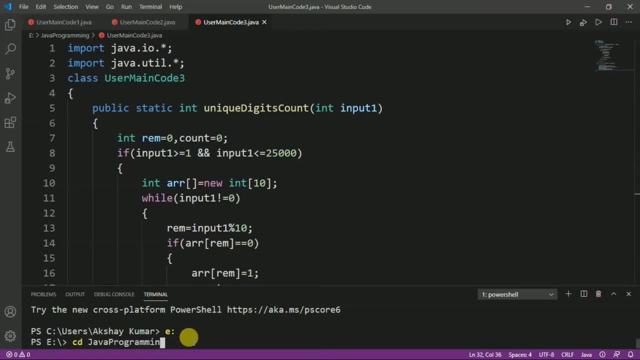 the folder Java programming. so let's go into the Java programming folder and now to run this, we have to write the following command: javac, with file name, that is user main code 3, dot. Java, and let's press Enter you, and now we will write Java, user main code 3 here. one message has came out. 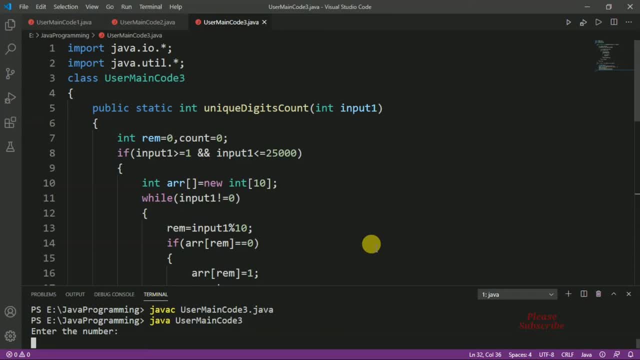 enter the number. so let's take the number which has given in the question. so let's take 292, and here we can see that there are two unique digits, that is, 2 & 9. so our program should return 2. so let's check, and here we can see that it. 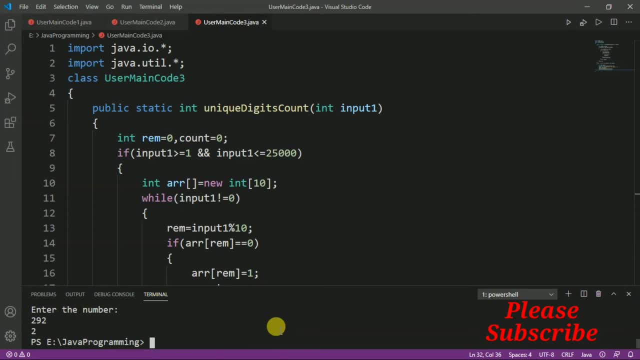 returns 2 and let's run the program for another input. so this time we will take the another input which has given in the question. so let's take 1015 and here we can see that there are three unique digits in this number, that is, 1, 0 & 5. so 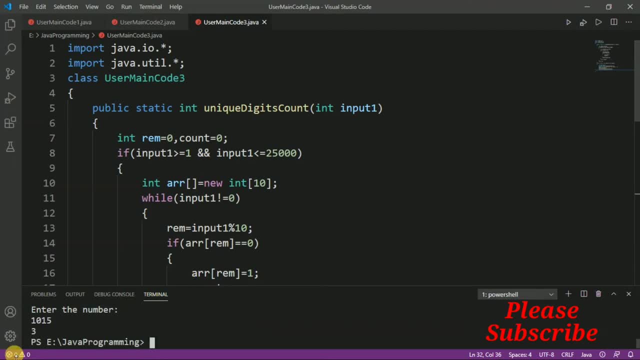 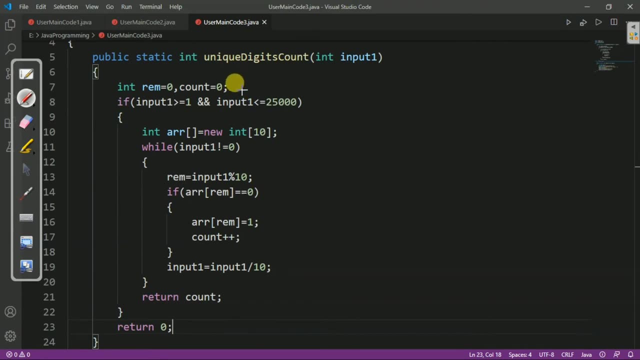 our program should return 3. so let's check. and here we can see that it returns 3, so it's correct. so now we will see how it works. initially we have to find the function named as unique digits count with one formal argument as an input, that is, input 1. so let's pass the value of actual argument which is stored. 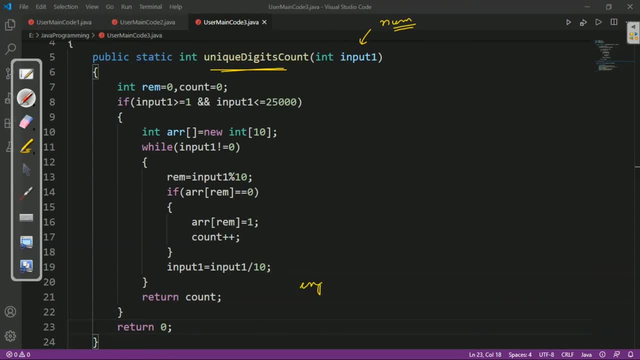 in the num variable. and so let's take input 1, equal to 1, 0, 1, 5, which has given in the question, and here we know that there are three unique digits in this number, that is, 1, 0 and 5, so our program should return 3, so let's check and after: 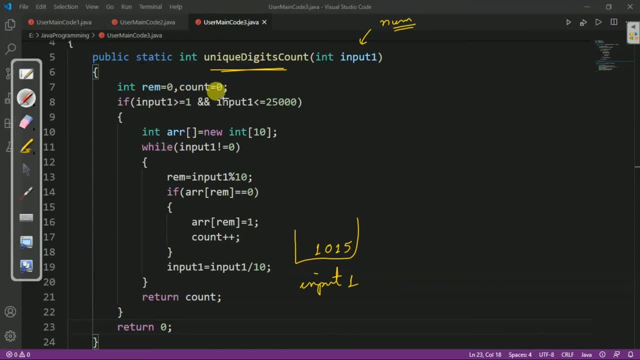 that we have initialized the rem and cont variable to 0. so let's take rem and initially the rem is for remainder and initially the remainder value is 0 and the another is cont and initially cont value is also 0, and after that we have written the condition for taking the inputs which should be in: 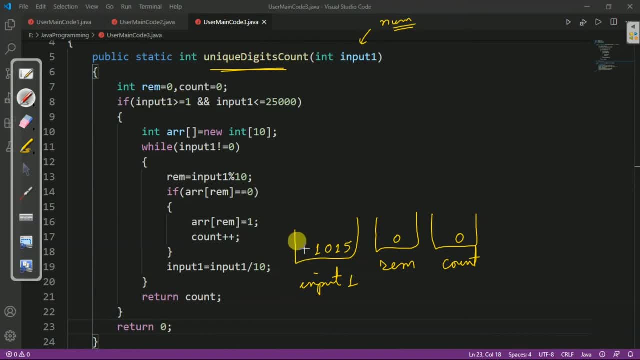 the range 1 to 25000. so let's check here. we can see that our input 1 is 1, 0, 1, 5, which is greater than 1 and less than 25000.. So this condition is true. So we will enter. 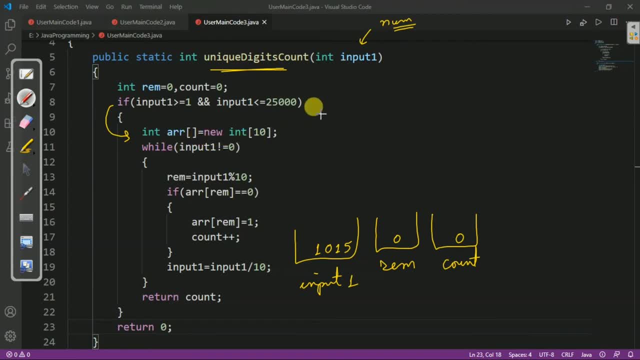 into this and after that we have taken the array of size 10.. So let us write here array of, let us create the box for the 10 elements, So 1,, 2,, 3,, 4,, 5,, 6,, 7,, 8,, 9 and 10.. So 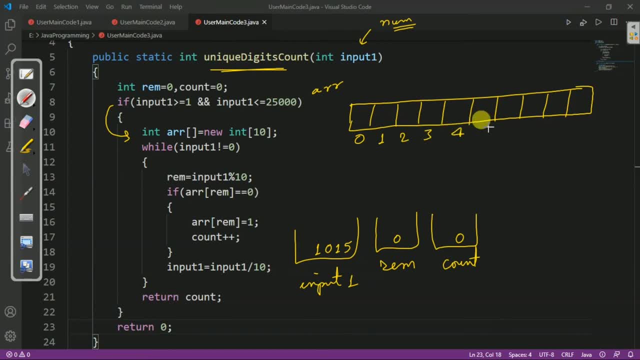 let us give the index 0,, 1,, 2,, 3,, 4,, 5,, 6,, 7,, 8 and 9, and here elements in the array allocated by this new will automatically be initialized to 0 for numeric type. So let 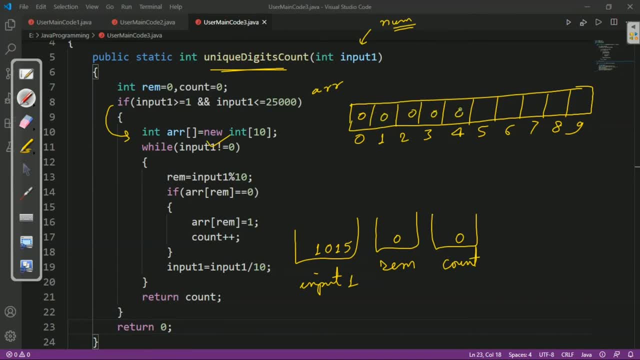 us put all the elements to 0, and after that we have taken the while Voilà loop and will take the condition while input 1 is not equal to 0, and here we can see that our input input 1 is 1015, which is not equal to 0. So we will enter into the loop and we will perform. 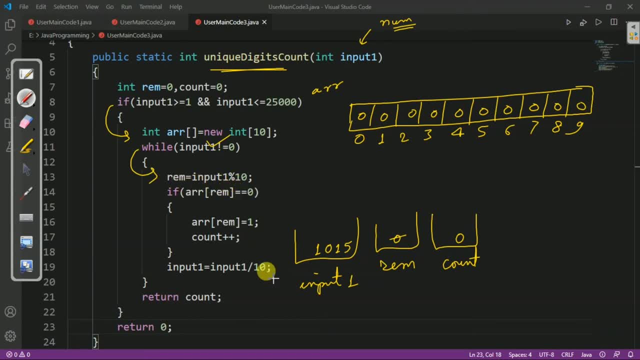 this operation REM equal to input 1, modulus 10.. So our input 1 is 1015 and modulus 10, it will return 5 and we will store that 5 into the REM variable. So now REM value becomes 5. 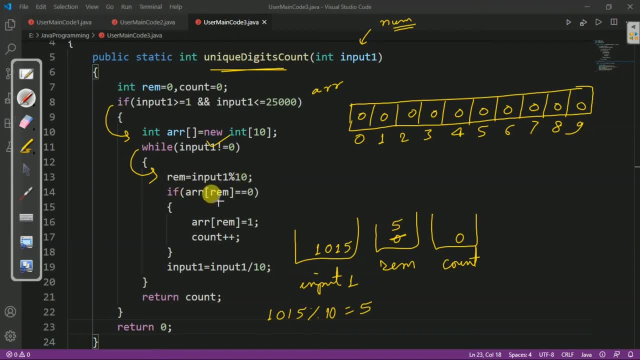 and after that we will check the condition. if error of REM equal to equal to 0- and here we can see that error of remainder means REM is 5.. So error of 5 equal to equal to 0, and here we can see that error of 5 is 0. So this condition is true. So we will perform this operation. 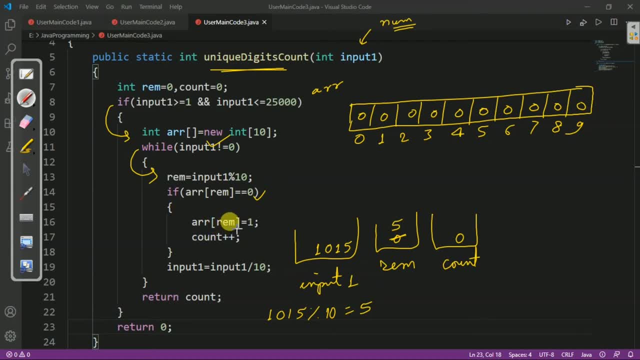 error of remainder equal to 1 means error of 5 equal to 1.. So now it becomes 1 and we will increment the count. So now count becomes 1 and after that we will perform this operation: REM equal to equal to 0, and here we can see that error of remainder is 5.. So 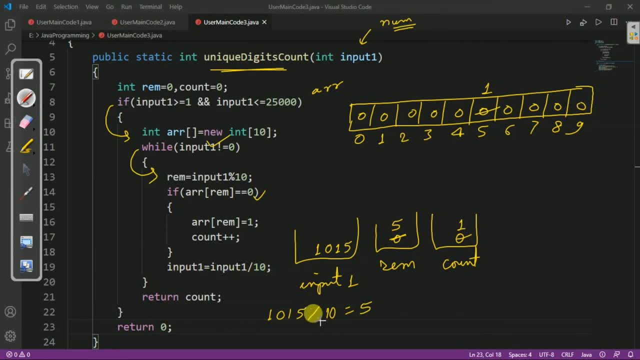 operation: input 1 equal to input 1 divided by 10.. So here 1 0, 1, 5 divided by 10. now it becomes 1 0- 1, and after that we will again check the condition here. while input 1 is not equal to 0, 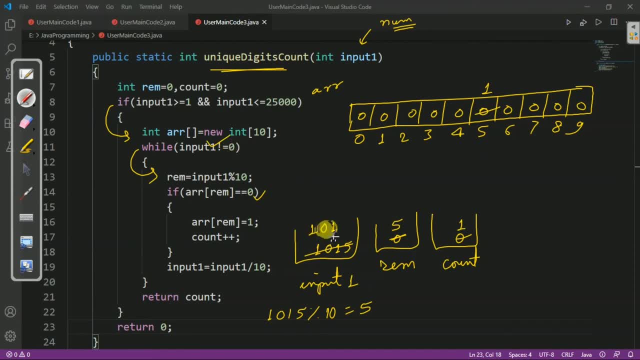 and here we can see that our input 1 is 1, 0, 1, which is not equal to 0. So the condition is true. So we will again enter into the loop and perform this operation, and this time input 1. 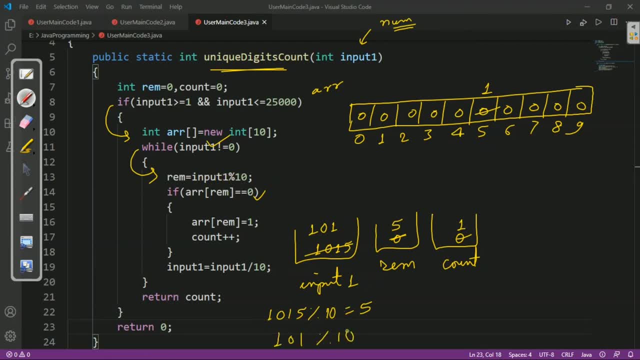 modulus 10.. So 1 0, 1, modulus 10, it will give 1 and we will store that 1 into the REM variable. So now REM becomes 1 and now we will check the condition if error of remainder equal to equal to. 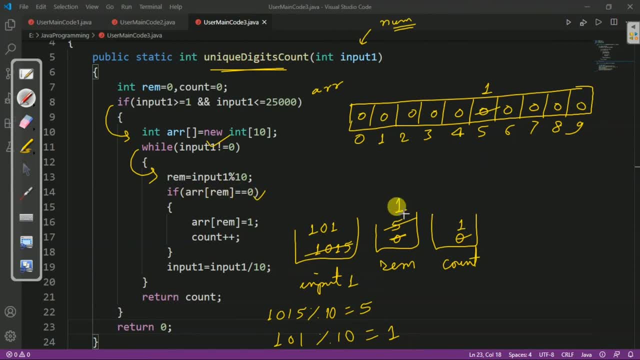 0, and here we can see that error of REM means error of 1 is equal to 0 or not, and here we can see that error of 1 is equal to 0. So this condition is true. So we will enter into this. 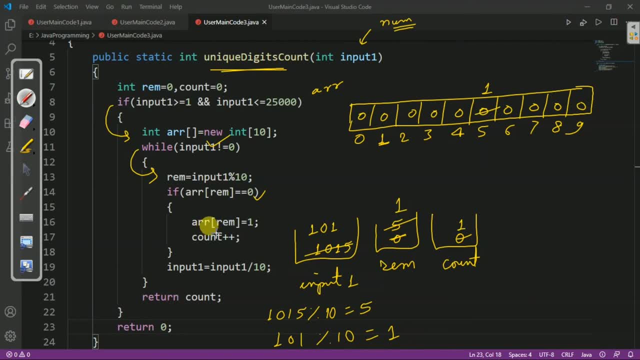 statement and We will perform this operation. error of REM equal to 1.. So error of 1 becomes now 1.. So here it will be updated to 1, and now we will increment the count, So this time count becomes: 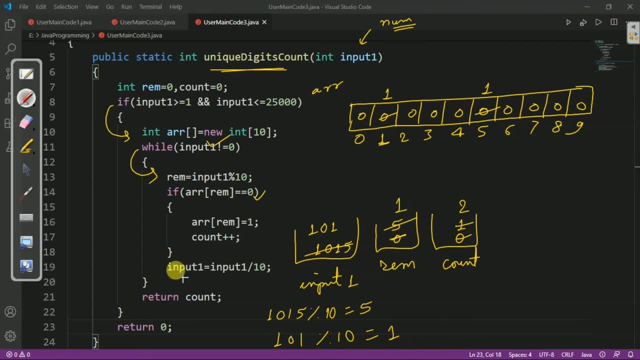 2. and now we will perform this operation again: input 1 equal to input 1 divided by 10.. So here, 1 0, 1 divided by 10. now input 1 will be updated to 10, and again we will come here and 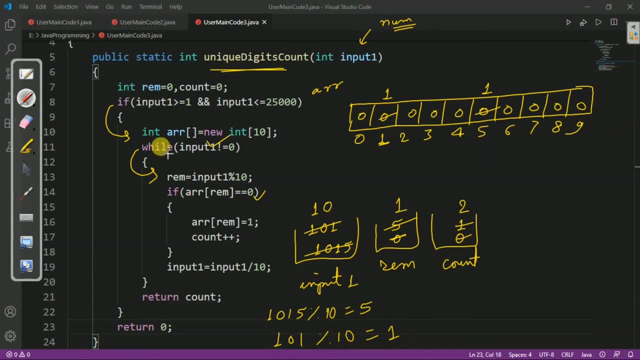 we will check the condition. while input 1 is not equal to 0, and here we can see that our input 1 is 10, which is not equal to 0. So the condition is true. so we will again enter into the loop and perform the. 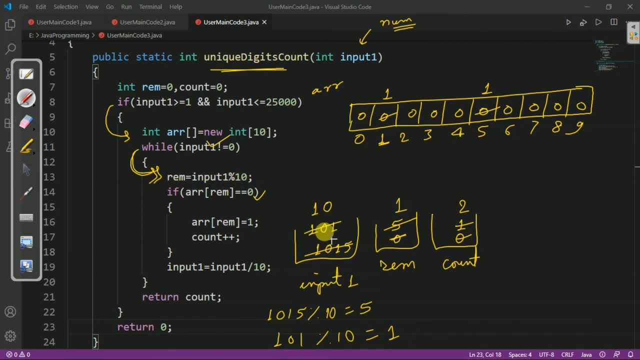 operation: REM equal 2. input one modulus 10. So here our input 1 is not 10, so 10 modulus 10 it will give 0. So we will store that 0 into the REM variable. So here REM becomes now 0, and after that we will check the condition if error of REM. 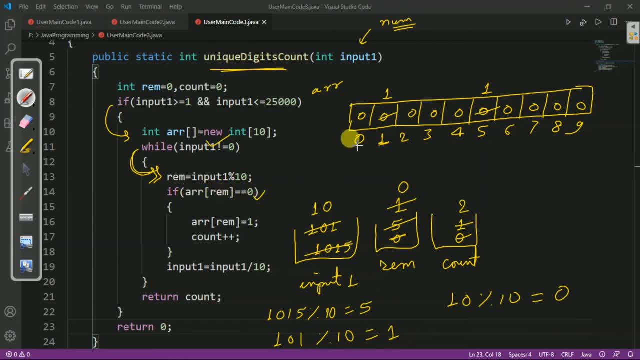 equal to equal to 0. and here we can see that error of 0 means error of 0 is equal to 0. So the condition is true. So we will perform this operation. error of remainder equal to 1.. So here error of 0 becomes now 1.. 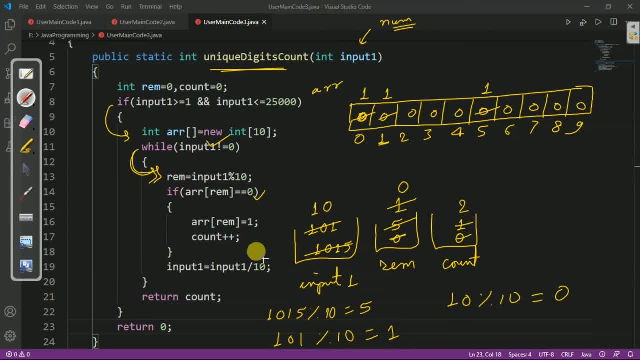 So here error of 0 now becomes 1, and after that we will increment the count. So now here, our count value becomes 3, and again we will perform this operation. input 1 equal to input 1 divided by 10.. So here input 1 is 10 and 10 divided by 10. now it will give 0, and now we will again check. 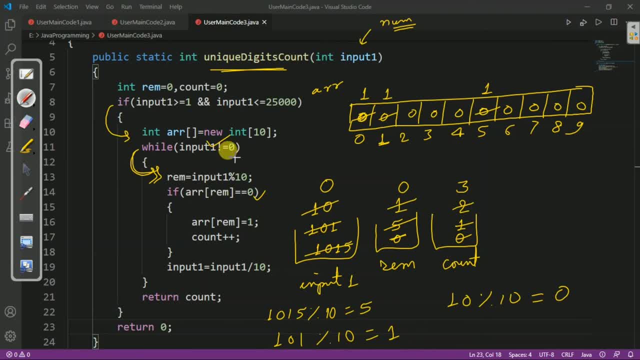 the condition while input 1 is not equal to 0, and here we can see that our input 1 is 0. So this condition will false and we will come out of the loop and we will return the count, And here we can see that our count value. 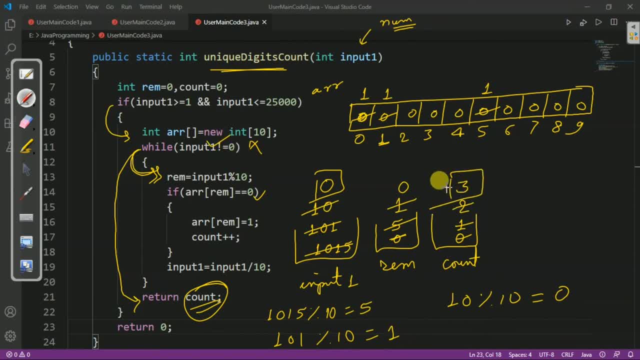 So our program will return 3 and we know that the in 1015 there are 3 unique digits, that is, 1, 0 and 5.. So it is correct. So please do like and share this video and subscribe our channel for more updates. Thanks for watching.